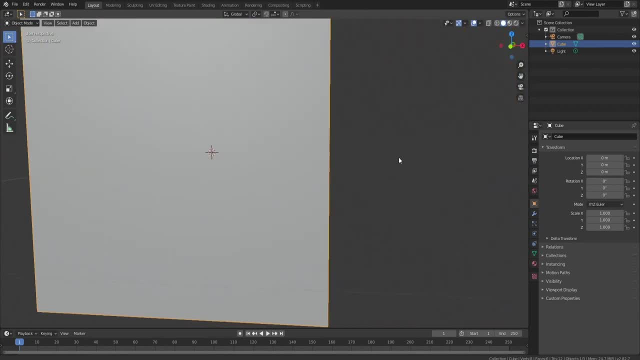 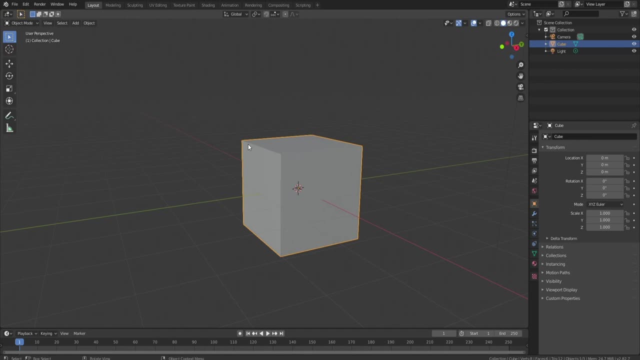 And your middle mouse wheel and kind of scroll through to see everything, So that, right, there is pretty much all movement is in Blender, just mouse wheel and mouse. That's it, guys. So to fly around you can press shift and F and that'll put you in this free cam mode and then you can use WASD to kind of go around wherever you want to look into it. I don't really use this that much. I used to use it a lot when I was starting out. That's the only reason I'm mentioning it, because it might help you. 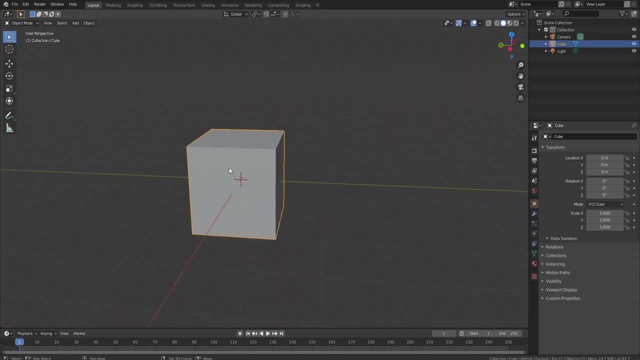 It might help some people. But after you get down the actual like mechanics of moving, I don't think you'll really be using that too much, because there's just so much. it's so much easier and faster to just kind of whip around like this. Now in Blender there's something called orthographic views- I think that's how you say it, And if you have a number pad on your keyboard, if you press one you'll flip straight to this front orthographic. If you press three, you'll go to the right. Seven is the top and nine is the bottom. So that's kind of how you. 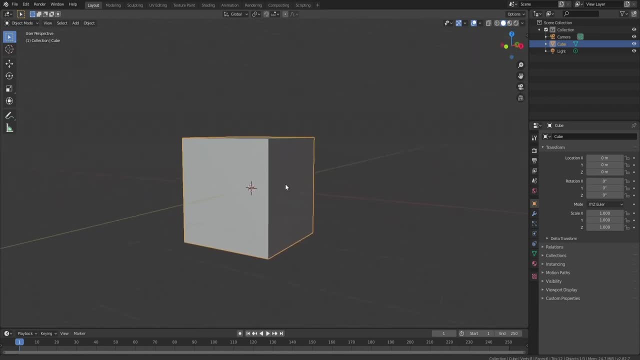 use those If you want to know. if you do not have a number pad on your keyboard, you can hold alt and your middle mouse wheel down and kind of scroll over. So right now we're on the right. If we scroll over this way, we're on the front. If we do it again, left back, If you go like this, top and bottom. So if you use alt and press down your middle mouse wheel, you're going to be all good, all good to go and you don't need a number pad. So I think that is everything for the movement side. 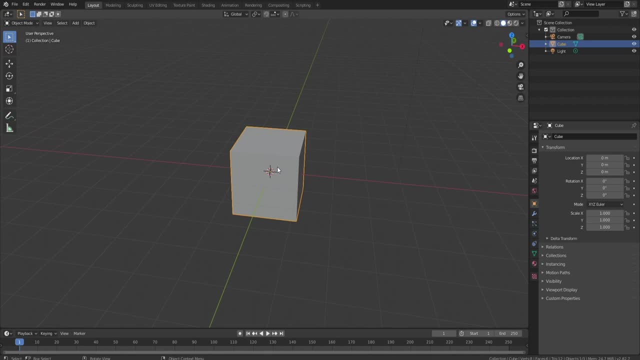 of things in Blender. I kind of stumbled my words, but it's all good, I'm trying out here. Up next, we're going to go into the modes. The only two modes you really need to know as a beginner is edit mode and object mode. Right now we're in object mode and we can do things like scale this if we want to. That's about it, though If you press tab on your keyboard, you're going to go into something called edit mode. Now, as you can see, all the vertices which are these points here are like a bit darker of an orange, which means those are higher. 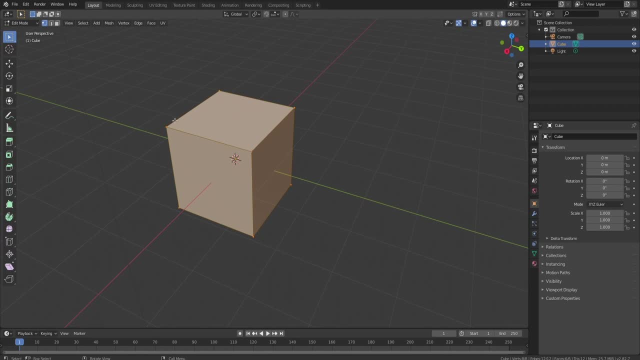 highlighted, You have three selection modes you can use in Blender. There's a vertice mode, which we're on right now, Line select mode, which, as you can see it, selects the lines, or face select mode, which is probably the most used one by most people, unless you're doing a very, very detailed model Now. with that being said, we're going to be in this face select mode and there's really only a couple hotkeys that you're going to want to know and really there's only a couple that you're going to use overall in Blender. 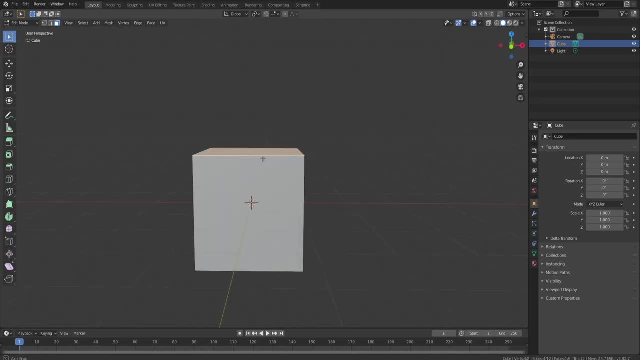 For most of your objects. the first one, and arguably the most important one in Blender is E. If you press E, it's going to extrude your object, giving you more of that object to work with. So now, instead of having only the one face, I can, you know, grab these and you know, move them how I want. So extruding is probably the most used one. and then S is the second for scale. So if you press S and then just move your mouse, you can scale. Now you can do. 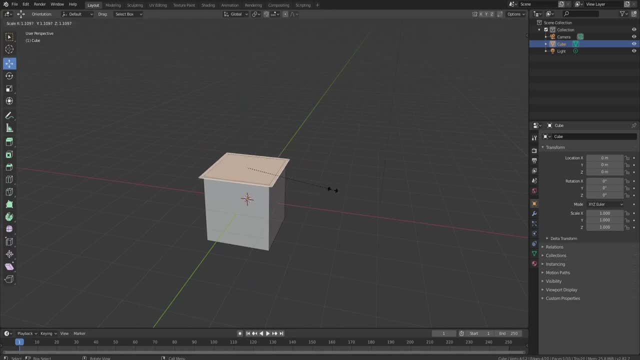 these up as well. So if you press E and then S, now you are scaling the extruded piece, So you're not scaling the normal face, you've extruded it, All right. So those are the main two hotkeys. There is a couple more that I'm going to go ahead and go over, though We have. let me go ahead and just mess this up a little bit. so it's not a perfect cube, So this will look a lot more demonstrable. There we go. We have R, which is rotate. 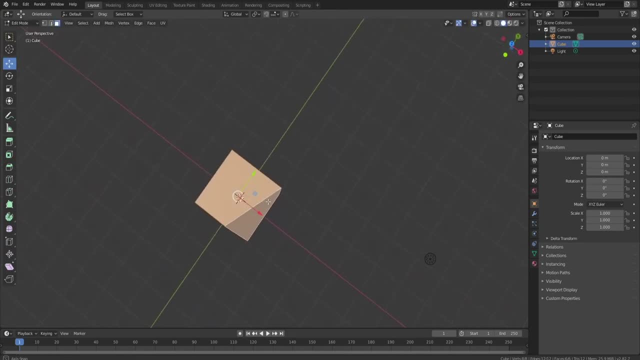 And it's as simple as it sounds. Now, if you're looking at this like in a weird angle, your rotate is going to be on a weird axis. But if you press R and then your direction- So right up here you can see- Z would move it up and down. So R and then Z, we're going to move on this axis. All right, And I use this little thing all the time because I always get confused, like oh, what button am I supposed to click? What way is what way? kind of a deal. So R and then any axis is how you're going to rotate. 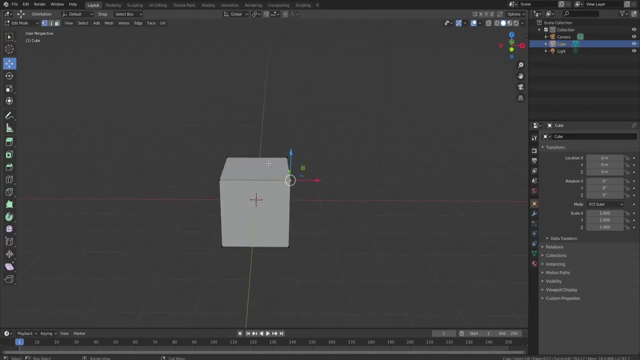 Along that axis, And you can do that with anything as well. If I wanted to, for example, extrude this, But I only wanted to extrude it on the X axis, I could put E and then X, And now, as you can see, it's locked on the X axis And you could do that with anything. if you want to scale and then press X, It's only going to scale on the X axis. S and then Y, It's only going to scale on the Y axis. This is going to be very helpful later on. 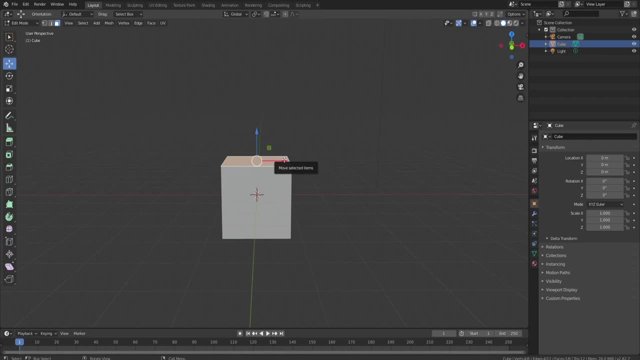 A very widely used one- but I don't use it that much. Apparently a lot of people do- is going to be G. If you press G on your keyboard it's going to grab, So you can kind of just move it wherever you want to move it. And then, of course, if you want to lock it on an axis, you can press G and then whatever axis you want to lock it on. Now, this last one, nobody really really uses it, But I do think it's important. Once I figured out about this I was like wow, that is a game changer And I don't know if it overly needs to be included in a super 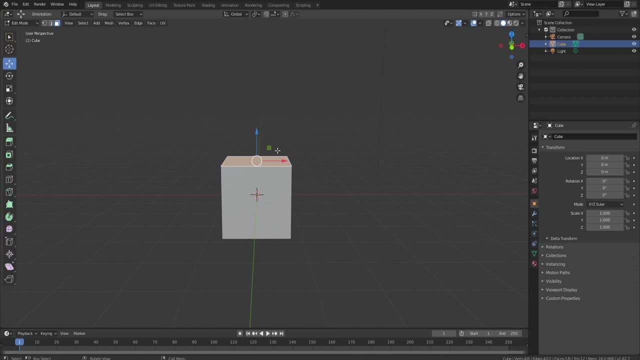 beginner tutorial, But it was awesome when I found it out, So I want to share it with you guys. And it's this guy right up here: Proportional editing. So you can just click on the button or you can press O on your keyboard And what this does is it pairs up with, for example, scale or grab. We'll use scale And let me add a couple loop cuts in here as well, Which is control R while you're in edit mode, And you can use your scroll wheel to go ahead and add more or less. We're going to add two of them, Since we have this proportional editing. 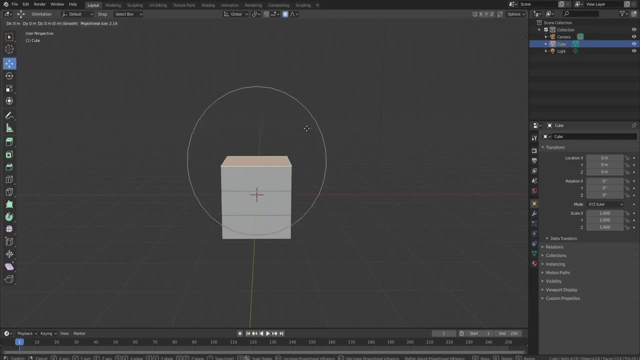 tagged on. If we were to press G, we have this little circle And we can use the scroll wheel to affect how much it's grabbing. So, as you can see, we have this, But if we scroll in on our mouse wheel it's not going to be grabbing as much. So this is very cool. Like, for example, if you made a whole tree, you can grab the top point of that tree and then add a curve to it at the end. Just something I thought was amazing Might definitely be confusing to new players- Or not new players- New modelers And last,